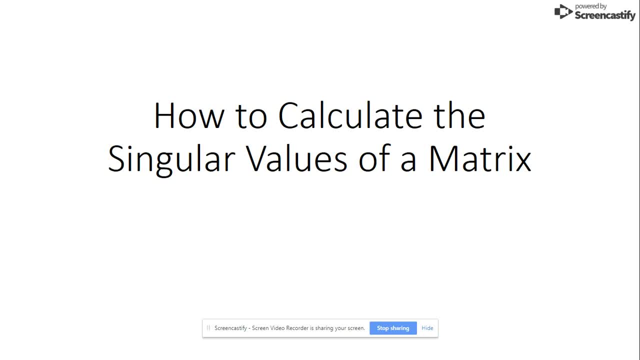 In this video we're going to run through how to calculate the singular values of a matrix, and this is actually really quite simple. So we'll start by going through the basic procedure and then we'll run through a worked example. So let's imagine we've got a matrix A and that matrix is a. 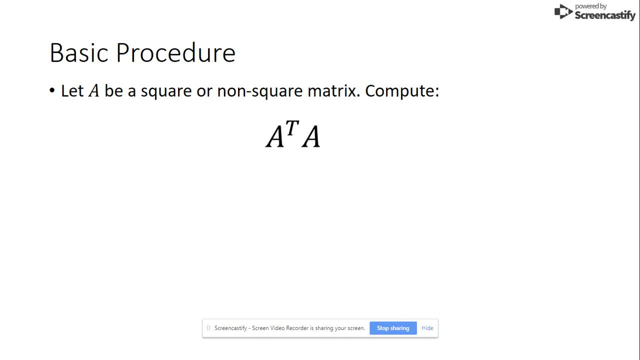 square or a non-square matrix, It doesn't matter. The first step is we calculate A, transpose A and that product will always, give, absolutely always, a square matrix and that means we can work out the eigenvalues, because we can't work out the eigenvalues of a non-square matrix. 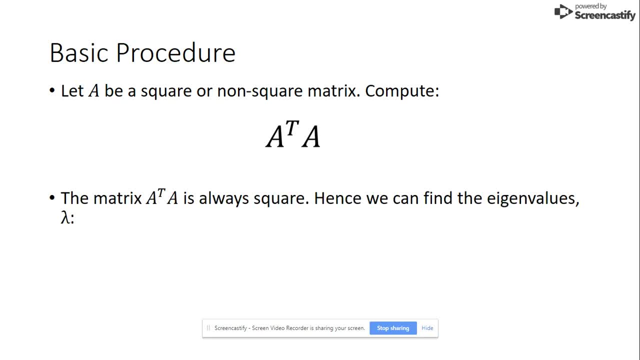 so that's why we have to do A transpose A. The next step is because we know that A transpose A is always square. we find the eigenvalues and, as is the normal procedure with finding the eigenvalues, we take the determinant If A transpose A minus. 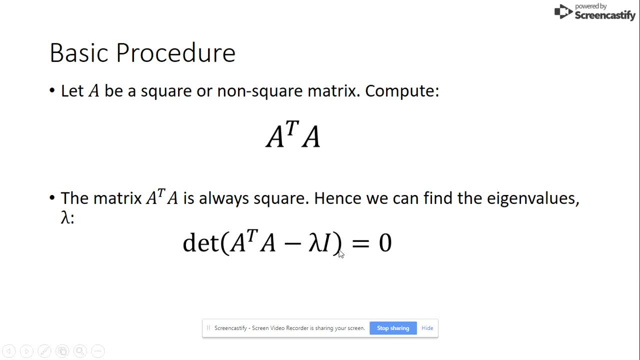 lambda, which is the eigenvalue multiplied by the identity matrix, and that is all equal to zero and that lets us form a polynomial which we can solve. And the singular values are found from the non-zero eigenvalues of A transpose. A Worth remembering non-zero and the way we take. 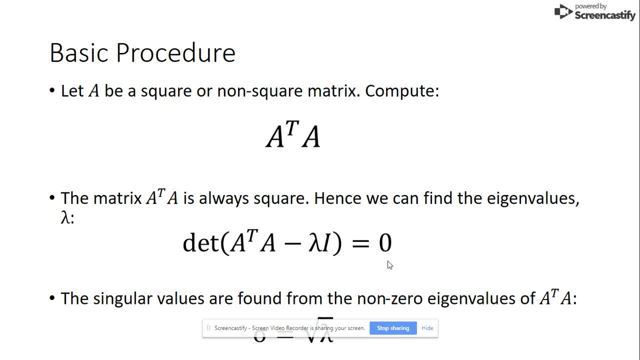 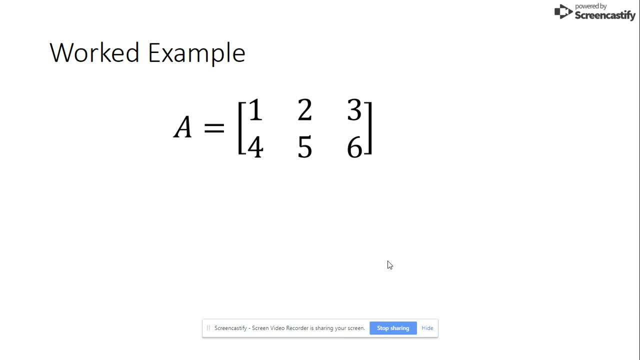 the eigenvalues and turn them into singular values is we simply find the square root of the eigenvalues. Let's run through a nice simple example. So we've got a 1, 2, 3, 4, 5, 6 matrix, and this is, of course. 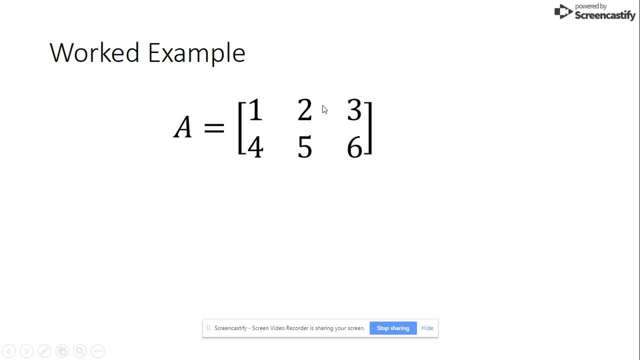 non-square because we have three rows and two columns so they're not equal, giving us a non-square matrix. So we start by finding A transpose A, which is just basic matrix multiplication. We've got 1 times 1 plus 4 times 4, which gives 17.. Then we do row times column, again getting 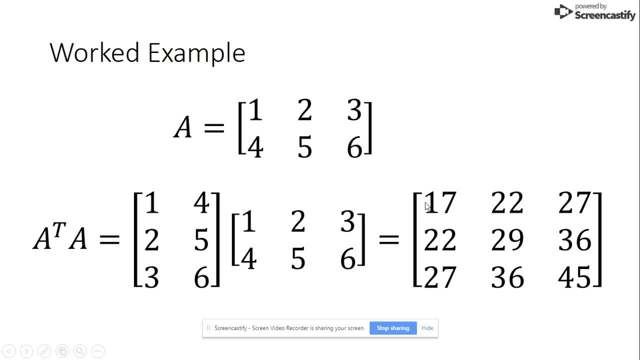 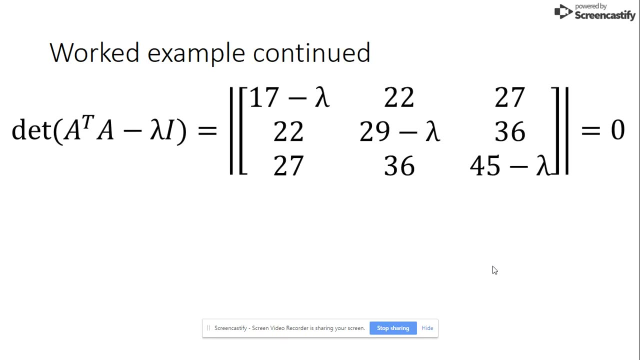 to 17.. And we follow that procedure through and we get A transpose A. We started with a non-square matrix and we've ended up with a square matrix of three rows and three columns. You've got N equals M, nice square matrix. We then take this matrix and we find the determinant of A transpose A minus.